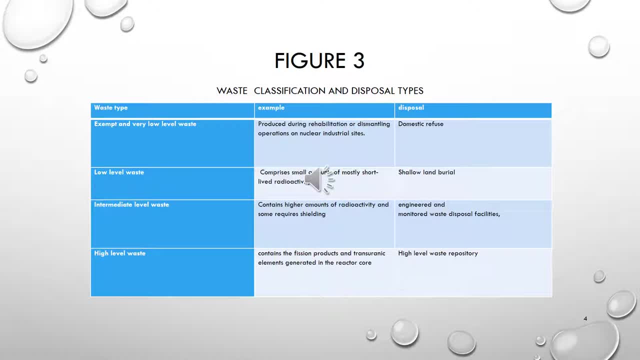 And then intermediate-level waste would be anything that contains higher amounts of radioactivity and some things that require shielding, And you dispose of that by engineered and monitored waste disposal facility. And the last is the high-level waste that contains sufficient products and transparent elements generated by nuclear waste disposal, And then you dispose. 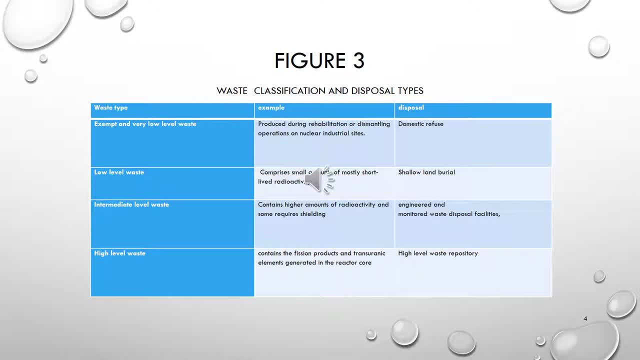 of that by engineered and monitored waste disposal facility. And the last is the high-level waste that are incorporated in a reactor core And you dispose of that with high-level waste repository, which is basically specified disposal sites. There are exempt and very-low-level waste. there is low-level waste, intermediate-level. 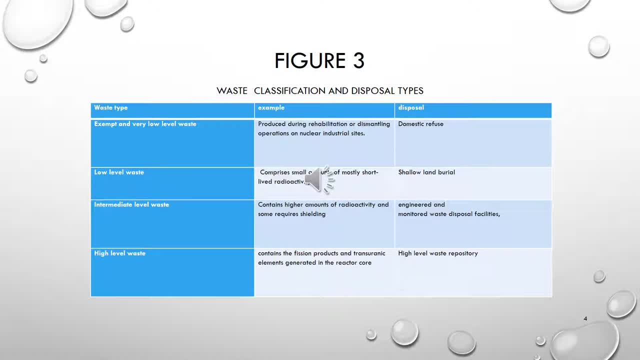 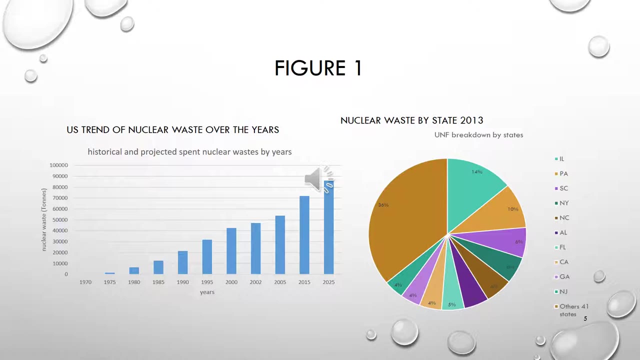 waste and high-level waste and the disposal mechanism goes according to the level of waste. you can see on the table the trend of with the historical project- this is a graph of a historical project- is spent nuclear waste by. yes, and as you can see, 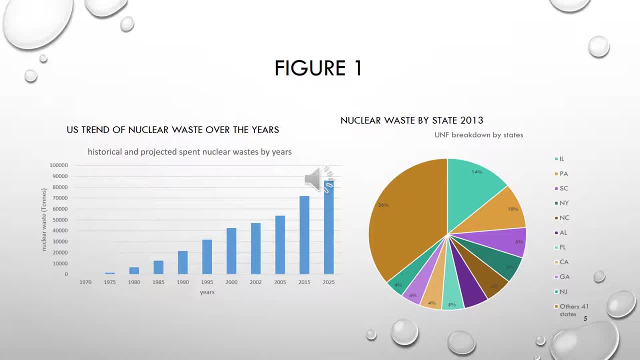 as is being going up and is projected to go even further off by the year 2025. and then there's also nuclear waste by State. for 2013- and you'll no- I had the highest nuclear waste, as you can say in a graph. and then the rest of the 10. 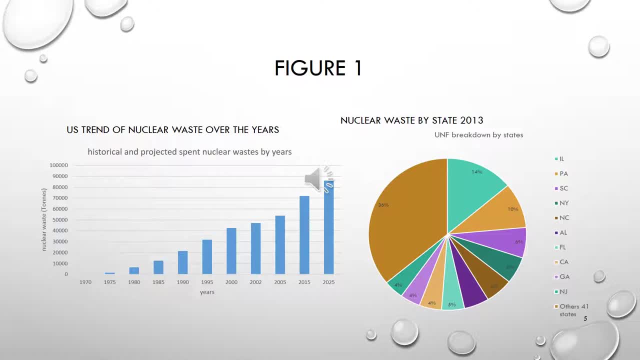 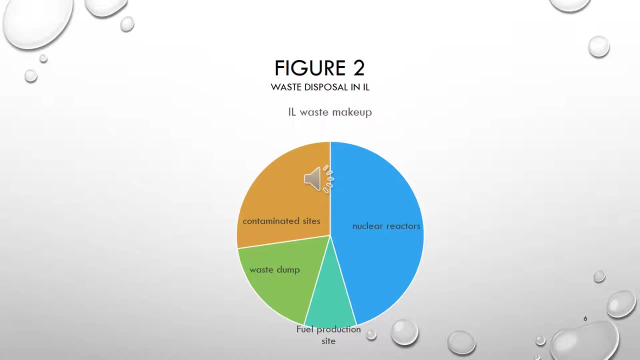 states have 64 percent of the waste and the rest of the 41 Tada's only had 36 seconds. Illinor has the highest, as you saw from the graph be on before they had. They have four reactors. they have three reactors that are closed, one that is not in operation. 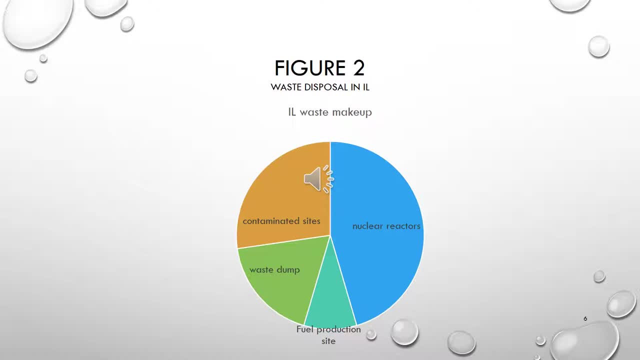 and six. that's working. And then they have waste. they have four waste zones, They have fuel production sites, they have research site center and then they have contaminated sites on three that are supposedly cleared up and then three that are still contaminated. 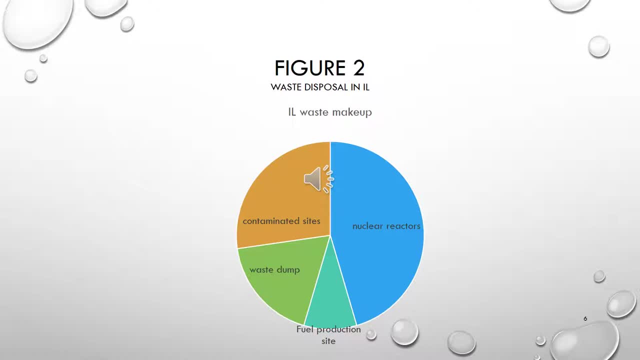 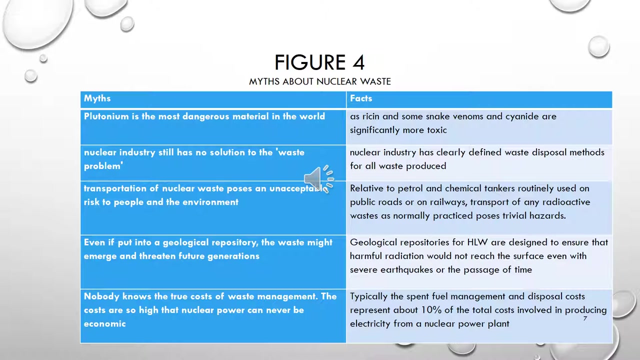 So they have a lot of nuclear activity going on in Illinois. That's why it has like a high nuclear waste on the graph. These are some myths about nuclear waste. For example, even if you put it into a geological repository, the waste by immersion 13 future. 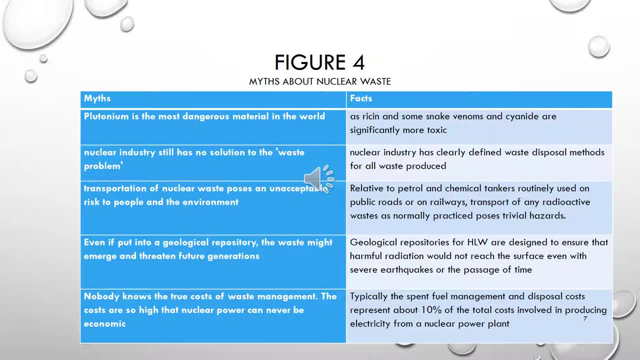 generations. that's not true. These repositories for high level waste are designed to ensure that how much of the waste is going to be in the future. So they have a lot of nuclear activity going on. in Illinois. They have four radiations that are not going to reach the surface even after a severe 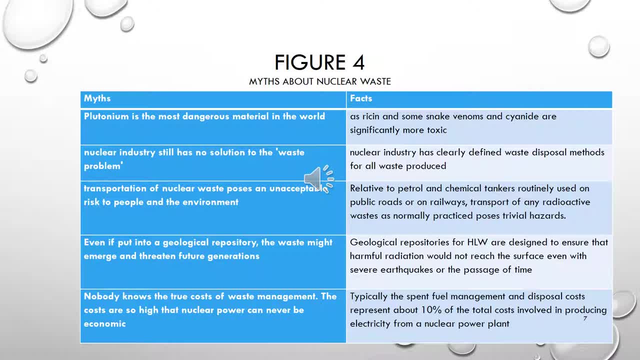 earthquake or passage of time. And then you have transportation of the waste, because it's an unacceptable risk to people and the environment. And that's not actually 100% true because, like the relative to petrol and chemical tankers, that's usually on the road. 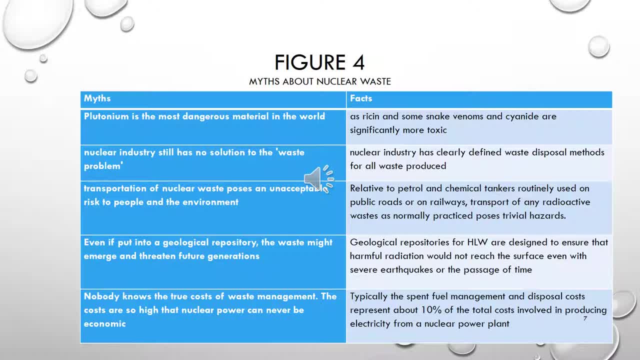 Radioactive waste that's normally practiced in the waste is normally practiced in places very, very far, very, very far away. So they have a lot of nuclear activity going on in Illinois. very small hazards, and then another one is the industry- have no solution to the waste. 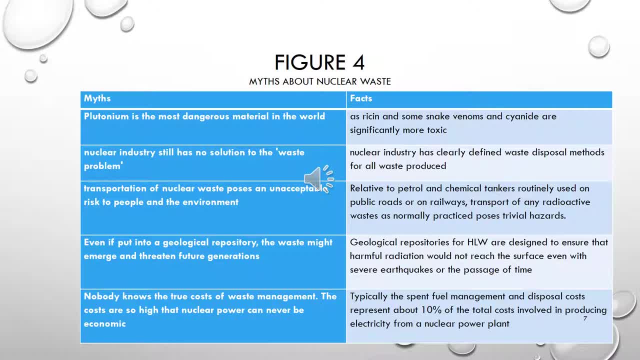 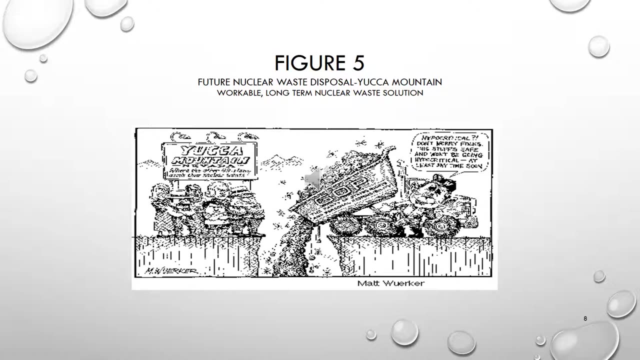 problem. as you saw from my presentation, that's not true. the industry actually have found different ways to manage the waste quote-unquote problem and it's proven so far this being implemented. so Yucca Mountain is a repository for high-level waste. that was supposed to be. 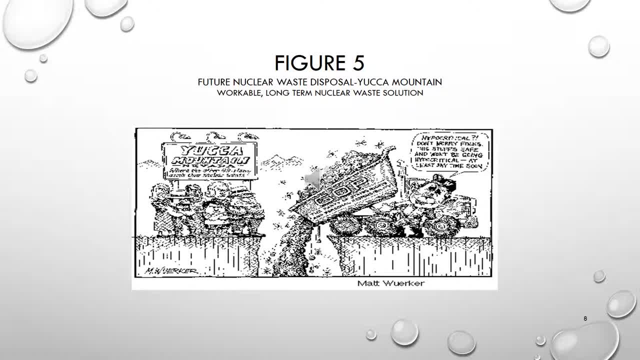 built and started. it's supposed to be a safely isolated use for about million years is. the project was initiated in the 1980s but due to protest from the community and back-and-forth legalities, it's currently not in action and it's not known if it's gonna go back to on to being you, if it's gonna ever be used. 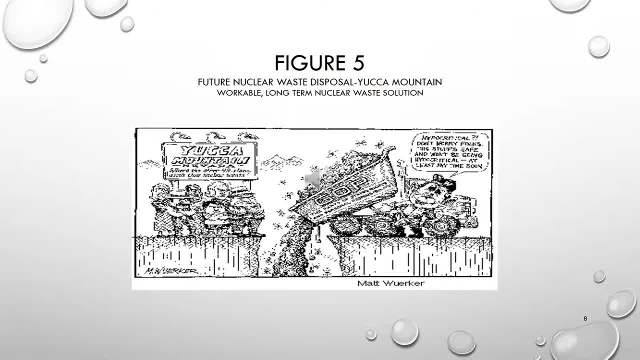 but it was supposed to be one of like the best ever reble 63 for high-level chemical ever build. and you know there's back and forth and whether it will, although I go through there's no. there know waste disposal tunnels receiving any facilities and there's no waste.